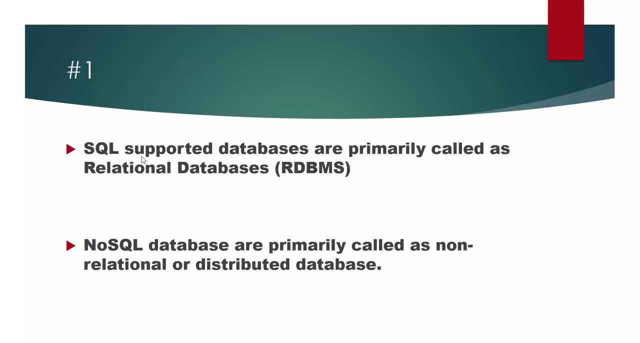 So let's come to the point. SQL separated databases are primarily called as relational database. SQL separated databases are primarily called as relational database. SQL separated databases are primarily called as relational database, which is our traditional database database, that is, the mysql and oracle. so no sql database are primarily called as non-relational. 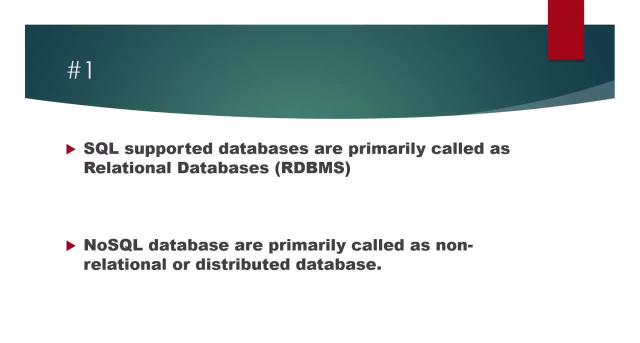 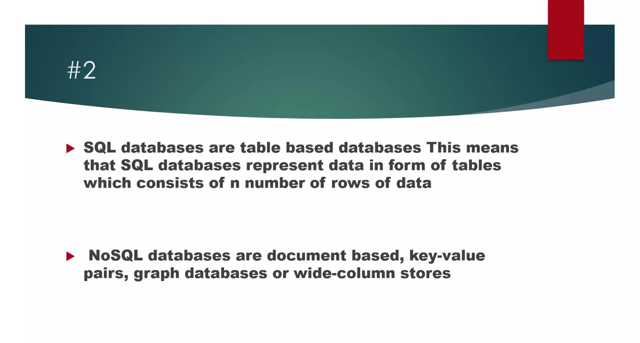 or distributed database. okay, so if anyone not aware on those no sql database which i mentioned- mongodb, cassandra, neo4j- already, i have uploaded tutorial on those database so you can check my tutorial. okay, so come to the next point. sql database are table based database. this means: 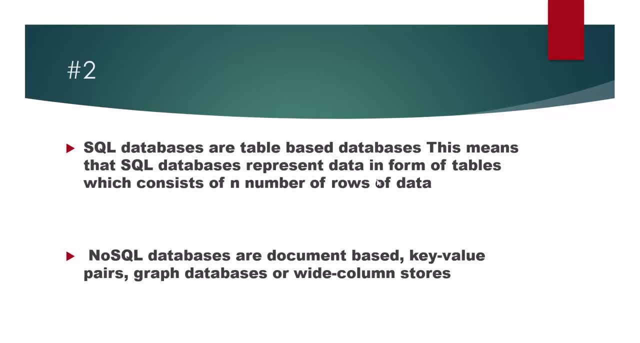 the sql database represent data in form of table which consists of n number of rows of data and each row we can say here as a object, and this table contains list of object. okay and no. sql database are document based key value pair. graph database are document based key value pair. 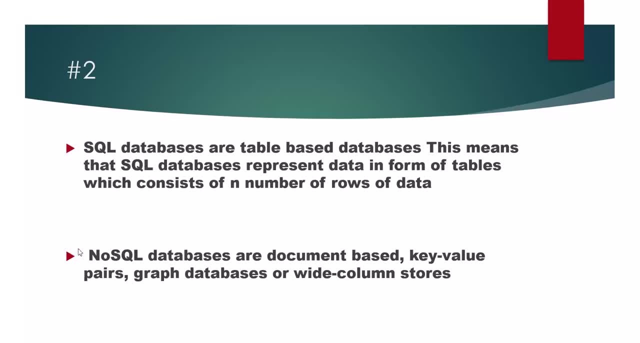 database or wide column stores. so if you observe here no sql database are document based. in mongodb database the data is inserted on format of document based and key value pair. and if you observe neo4j database, there we are storing data in the form of graph and in cassandra the data 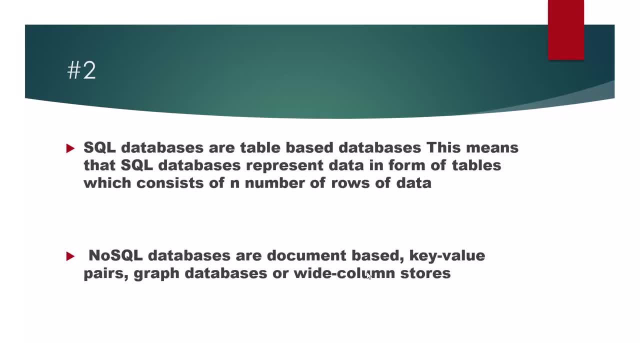 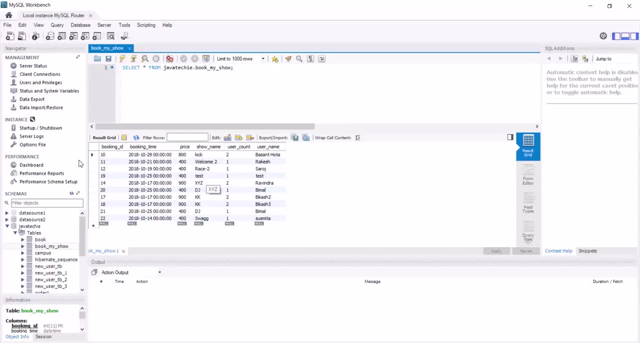 will store in the form of wide column. okay, so let me show you. so this is my rdbms relational database, where data is stored in part of table and having n number of row and this entire row we are calling is a object. okay, similarly, if you go to the mongodb, 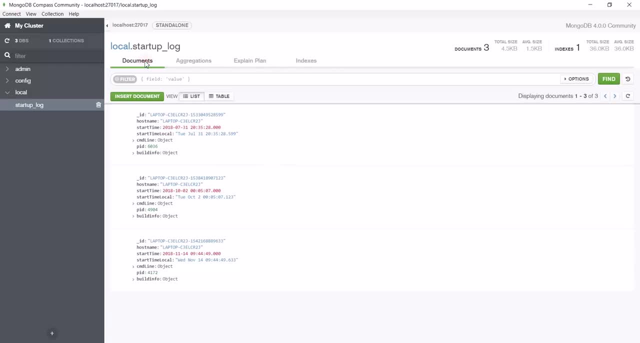 it's based on documents and the data in stored in the form of key value, pair, id. this is the key and value. similarly, key value okay, and neo4j. it will stored as a graph and in cassandra it will stored as a wide column so that it gives them more stability. okay, now let's move to the next slide: sql database. 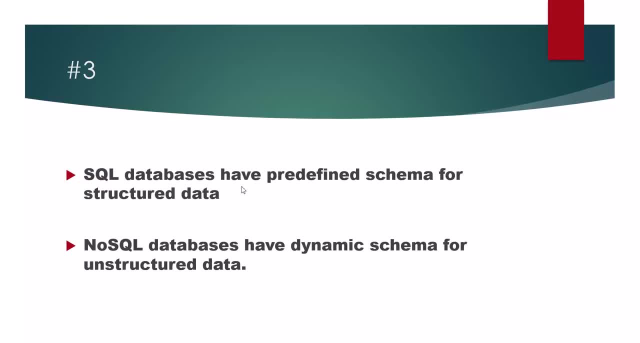 have predefined schema for structured data where no sql database have dynamic schema for unstructured data. so if you notice sql database have predefined schema for unstructured data. so if you notice in while we are doing any application using mysql, first we need to create the schema and we need 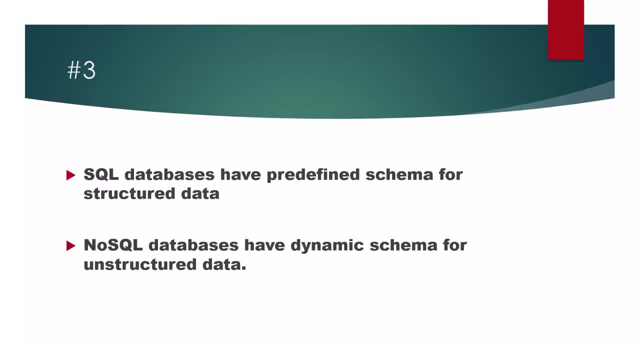 to do the data modeling, like the length of this field should be, like we need to mention that value and we need to specify. this should be not, not like this: we are doing the data modeling and we are creating the schema first. but if you observe, in no sql there is no predefined schema. 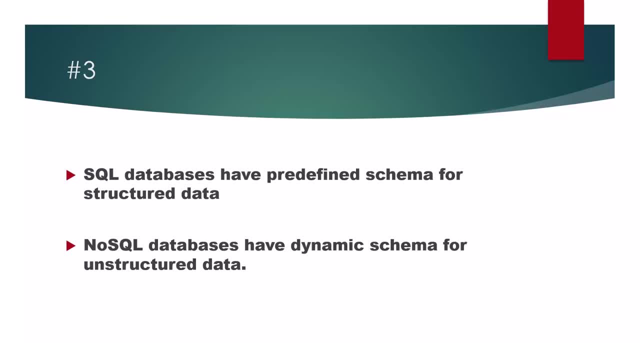 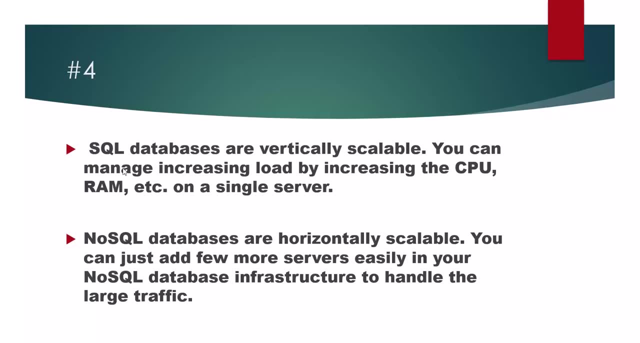 schema from our web application. we are generating the schema for no SQL database. ok, so SQL database are vertically scalable. you can manage increasing load by increasing the CPU, RAM etc. on a single server and in no SQL database are horizontally scalable, you can just add few more server. 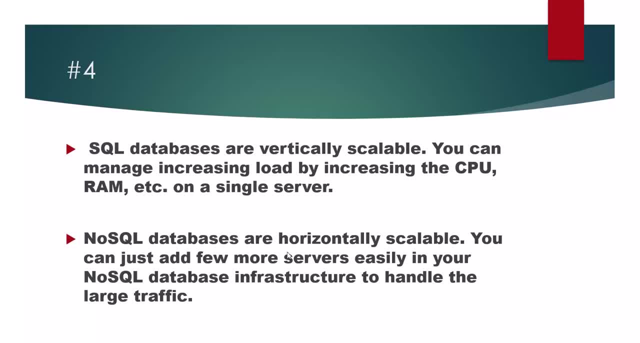 easily in your no SQL database infrastructure to handle the large traffic. so if on your database is getting more load then that will be easy to handle it. no SQL database to add few more node to handle the large traffic. in case of SQL we need to increase the horse. 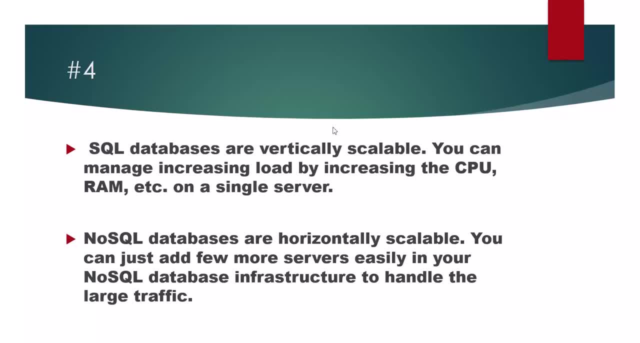 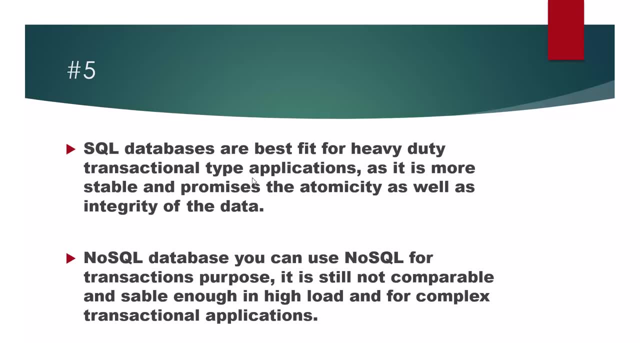 power of our CPU and RAM. SQL database are best fit for heavy duty transactional type application as it is more stable and promise the atomicity as well as integrity of the data. so no sql database. you can use no sql for transaction purpose. it is still not comparable and stable enough in high load for complex. 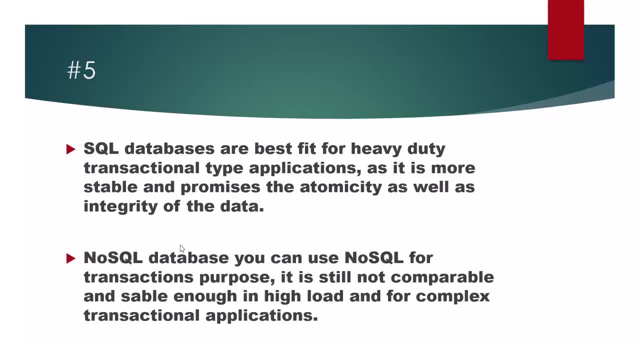 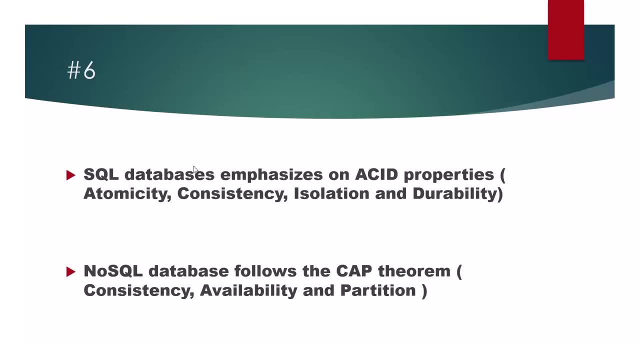 transaction application. so the moral here: sql database will support for the complex transaction business where no sql database will not able to handle that situation. okay, sql database emphasizes on acid properties, that is, atomicity, consistency, isolation and durability. but this no sql database follows the cap theorem, that is consistency, availability and partition. 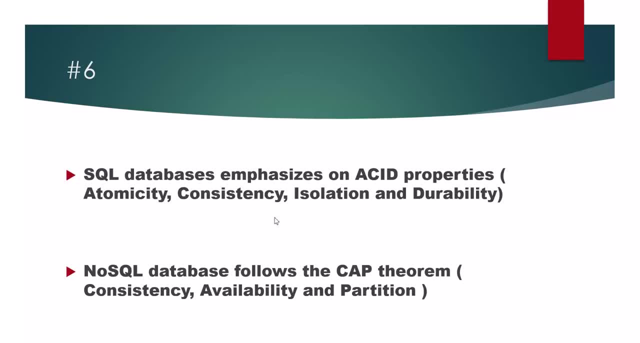 so for this, atomicity is our atomicity and transaction is our key role of our application. so if you want to implement the transaction as part of your project, we should not choose the no sql database because it was not able to handle the complex transaction as it is following the cap theorem. but it is good to use sql database if you have following the. 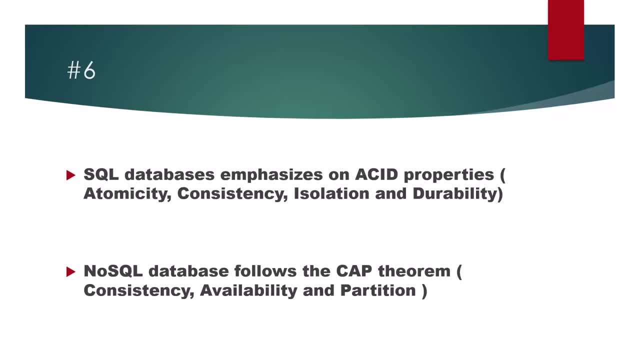 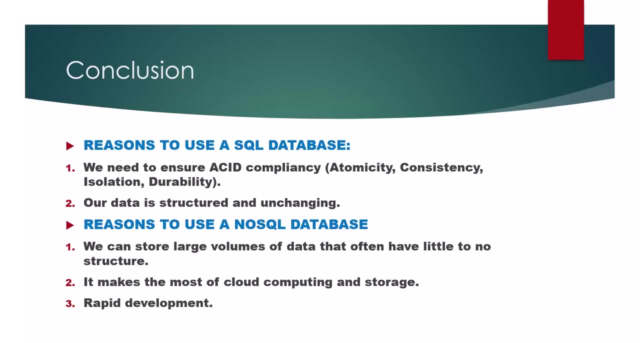 transaction. in case of no SQL also, we can apply the transaction, but for that we need to use the some design pattern, that is something like two PC, two phase commit design pattern, so that in no SQL we can go ahead for the multi transaction. okay, now let's go to the conclusion, so that we 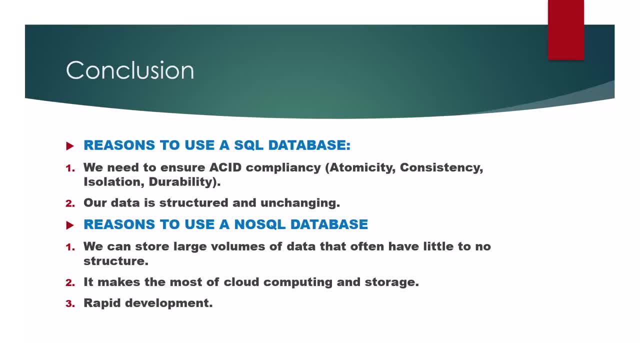 can identify which database is better and advantages and disadvantages of it. okay, so reason to use a SQL database. we need to ensure ACID compliancy, that is, atomicity, consistency, isolation and durability. our data is structured and unchanging. okay, if you want to achieve these. 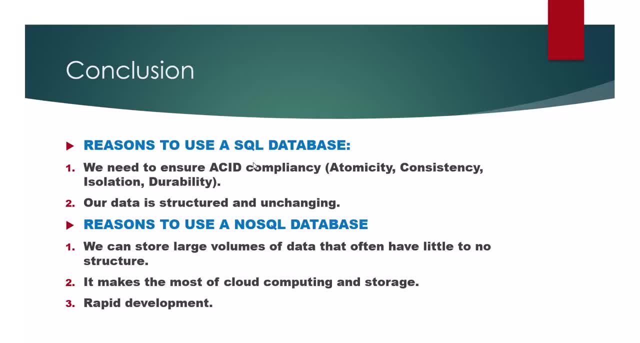 features. we should always prefer SQL database. reason to use a no SQL database? we can play with large volume of data with unstructured data. okay, it makes the most of cloud computing and storage and rapid development. so best use. I can say like if your application is monolithic. 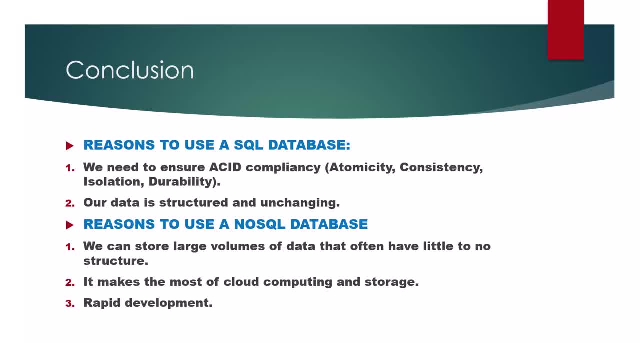 and it's deployed in local server, then we should prefer to use SQL database. if you are using micro service and you are deploying it any cloud platform, then we should choose the no SQL database. okay, and for retrieval purpose, as in no SQL database, data is unstructured format, it won't give the better performance, but in